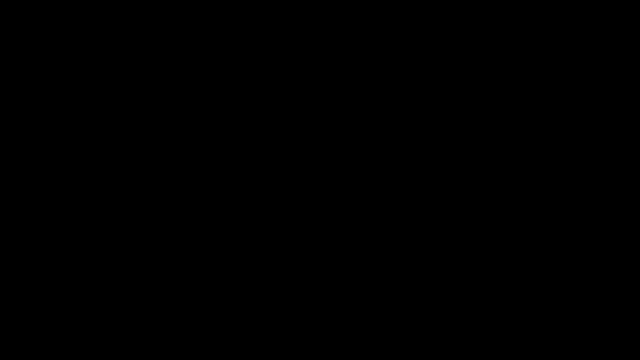 In this video I'm going to talk about orbital diagrams and how to draw them and how to place the electrons within each orbital. So let's start with nitrogen. So nitrogen has an atomic number of 7 and an average atomic mass of 14.01.. 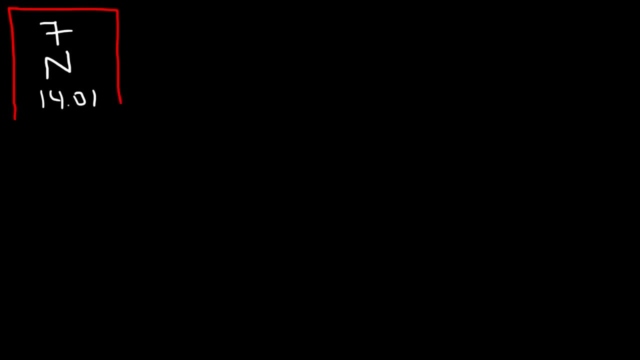 Now, in order to write the orbital diagram, or to draw it, first you need to identify the electron configuration of nitrogen. Now I've created a separate video on electron configuration. you can search for on YouTube. The electron configuration of nitrogen is 1s2, 2s2, 2p3.. So notice that the exponents have to add. 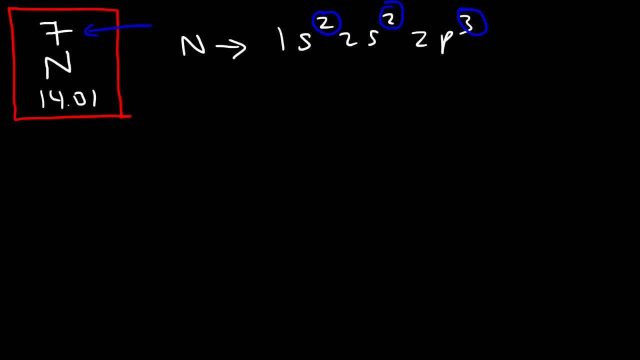 up to the number of electrons in a nitrogen atom. Now keep in mind: in an atom the number of protons, which is 7, is equal to the number of electrons In an ion. they differ. So once you have the ground-state electron configuration, then 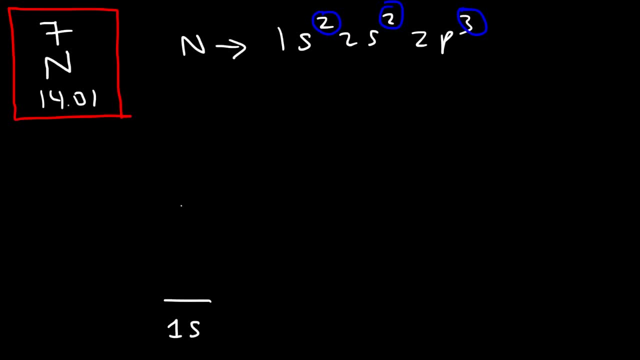 you can draw the orbital diagram. So this is the 1s energy level, this is 2s and this is 2p. P always have three orbitals. So what you want to do is you want to fill each orbital from the bottom all the way to the top. So the first orbital: 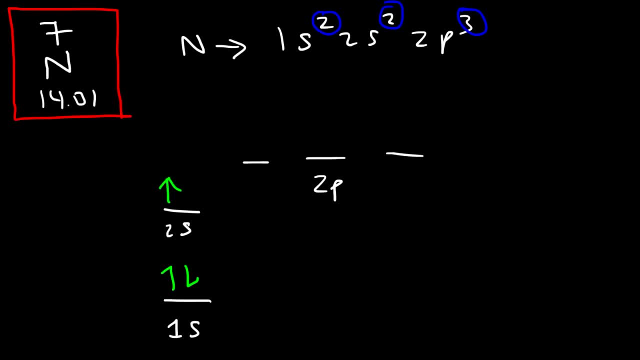 has two electrons, you need to put opposite spins. now, once we get to the 2p orbital, each of these orbitals, they have the same energy and so, as a result, they're known as degenerate orbitals. now, when you fill in degenerate orbitals, you need to fill. 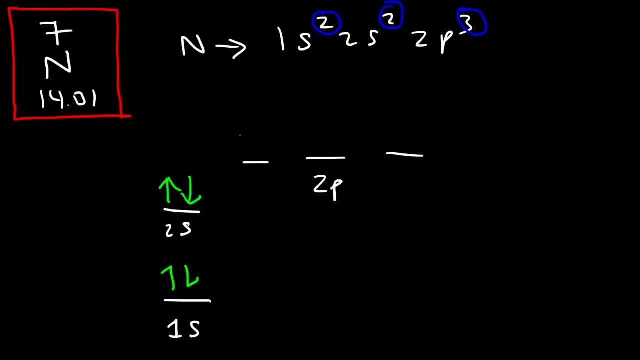 them up one at a time, with parallel spins. so once you put the first arrow in the first orbital, you should not put the second one in the same orbital. rather, the next one has to go in the next orbital, but with parallel spins. so if the spin is facing upward in this orbital, then the second spin should be. 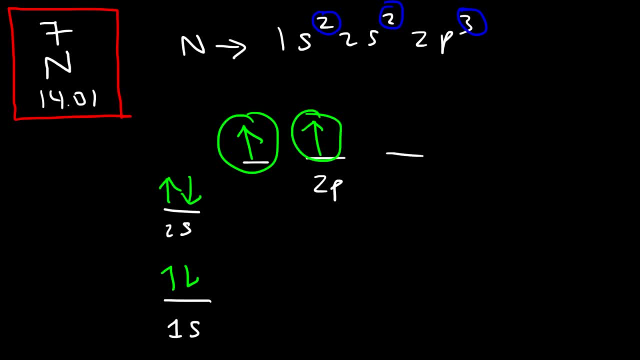 parallel to it, it should be facing upward as well, and the third spin will be doing the same thing. so nitrogen has three unpaired electrons. a substance with unpaired electrons is said to be paramagnetic, its weakly attracted to an external magnetic field. a substance that is composed only 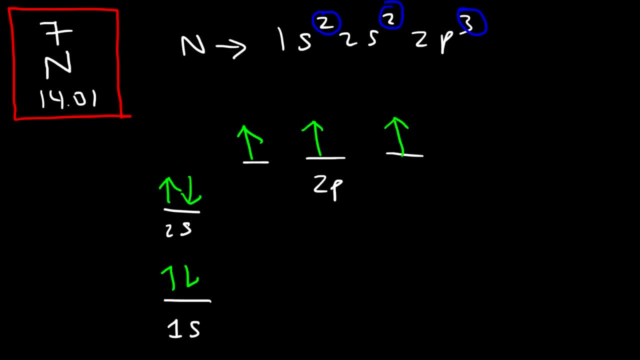 of paired electrons is said to be diamagnetic. it's weakly repelled by an external magnetic field, so nitrogen is paramagnetic. now I do want to make one small correction. I mentioned that you should write the electron configuration before filling the orbital diagram, and it turns out that you really don't need. 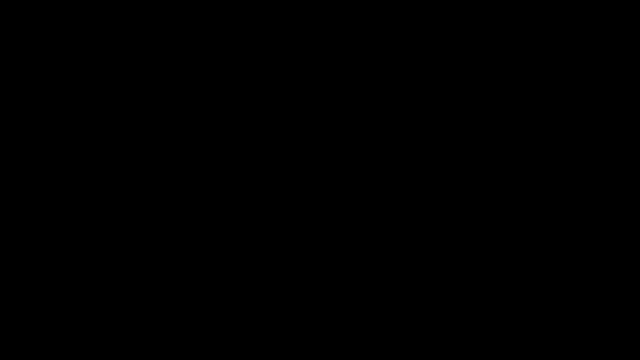 to write the electron configuration. if you want to, that's cool, but you don't have to, so I'm going to use magnesium as an example. it has a mass number of, or an average atomic mass, I believe, of 24.3, and the atomic mass is: 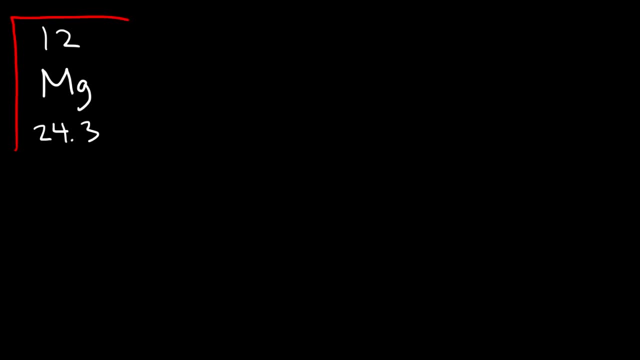 12. I mean the atomic number is 12. so an atom of magnesium has 12 protons and 12 electrons. so all you need to do is fill the orbitals until you reach a total of 12 electrons. so the first energy level is going to be filled. so that's two electrons. three: 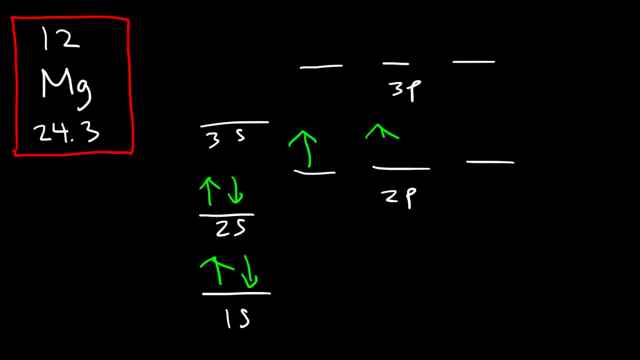 four, five, six, seven. don't forget to add electrons, one at a time, once you get to orbitals that have the same energy. so that's seven. we have eight, nine, ten, twelve and eleven. now to put the 12 electron. you don't put it here, you have to fill. 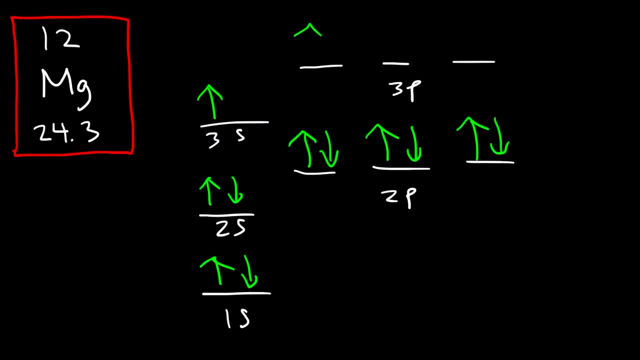 the lower orbitals first. so always fill the lower energy levels first before you jump to the higher energy levels. so this makes 12, and so that's how you can fill the orbital diagram of magnesium. now, if you want to write the electron configuration, you can literally see what it is is 1, s, 2, and then we have 2, s, 2, 2. 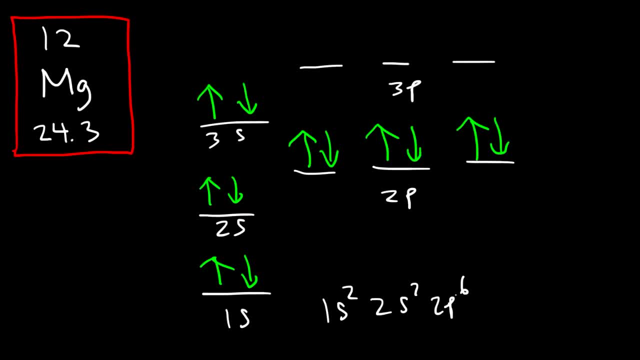 p 6 and then 3 s 2. so that's the electron configuration of the magnesium element. but, as mentioned before, you don't need to write that. you can just fill up the orbital diagrams until you reach a number of 12. so now it's your turn, go. 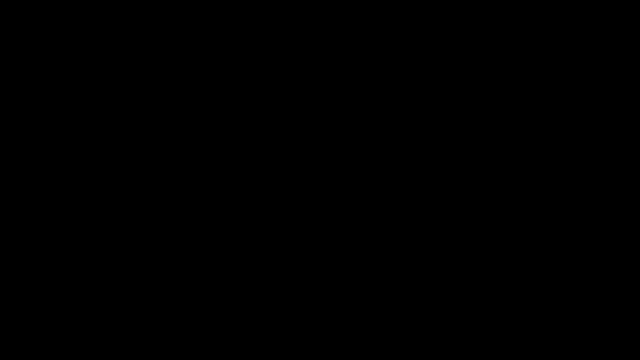